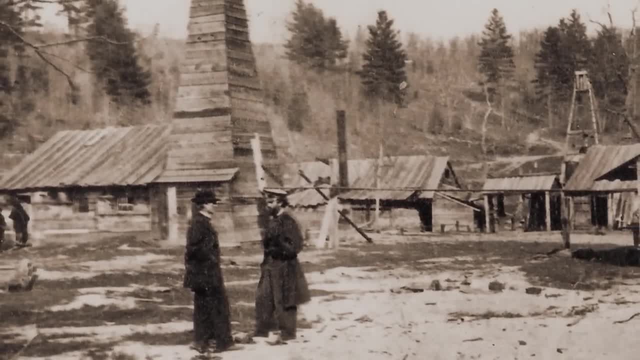 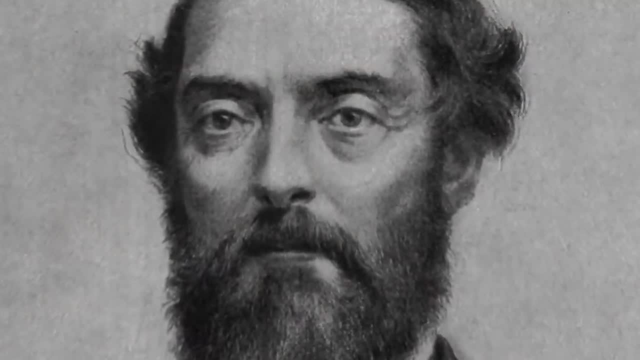 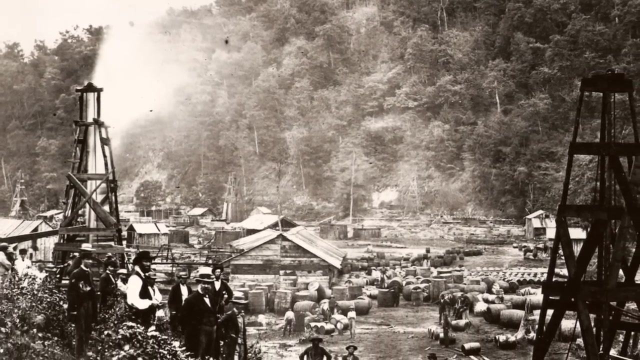 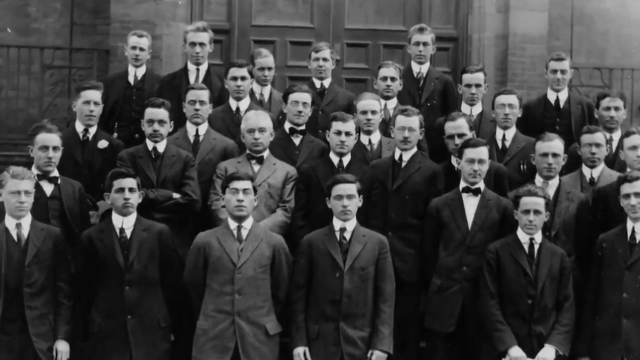 On an August afternoon in 1859, a former railroad conductor hired by the Pennsylvania Rock Oil Company drilled a hole 69 and a half feet into the earth and a whole new world sprang forth, A world made possible by chemical engineers with names like Brown, Walker, Olson and many others. 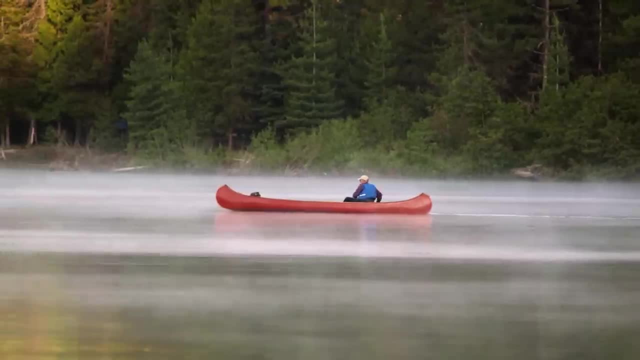 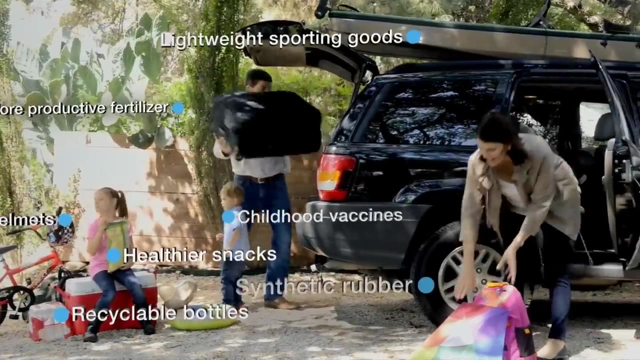 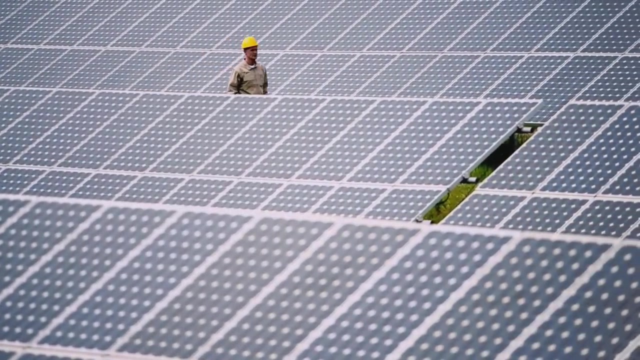 Like those who would follow, they saw the promise in the future. We live in a world that would be virtually unrecognizable without the contributions made by chemical engineers. Yet, for all the advances that have been made, the world has been made possible. 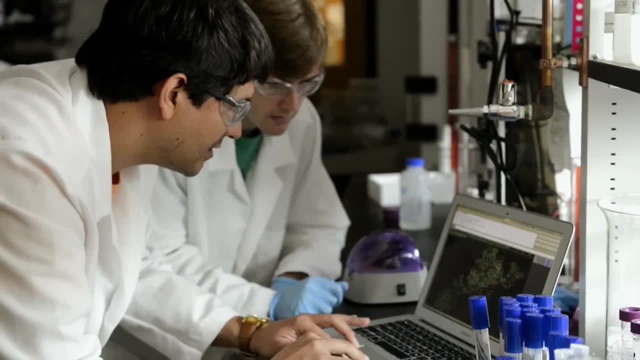 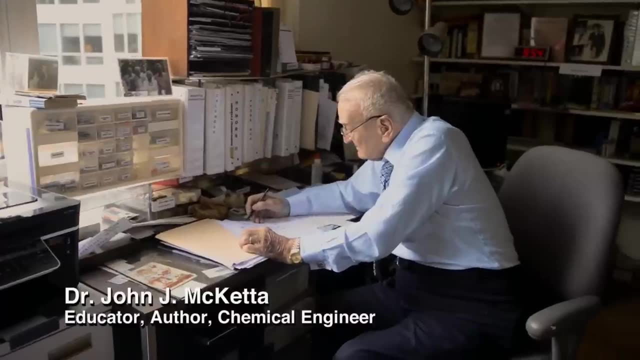 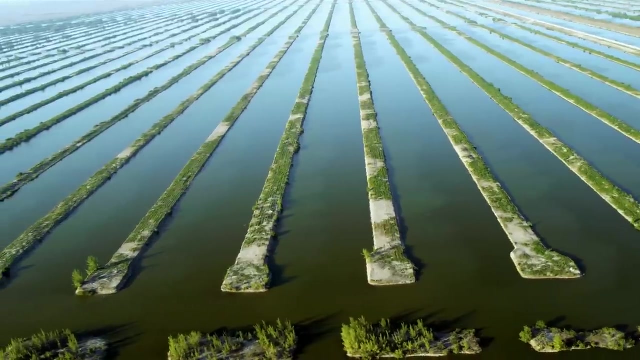 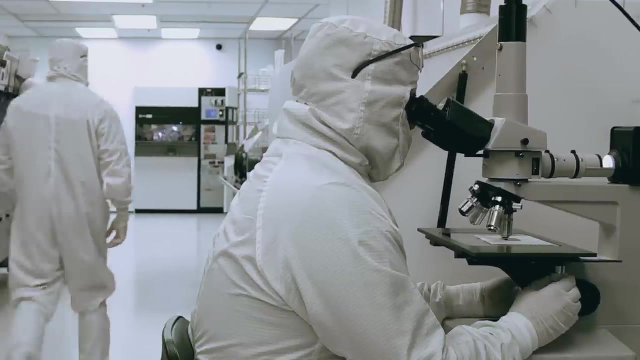 Challenges remain. Have we looked far enough ahead? Have we planned accordingly? In moving forward, there will always be unseen risks, dangerous processes, unwanted byproducts. What we leave behind are not just the advances we've made, but how responsibly we've made them. 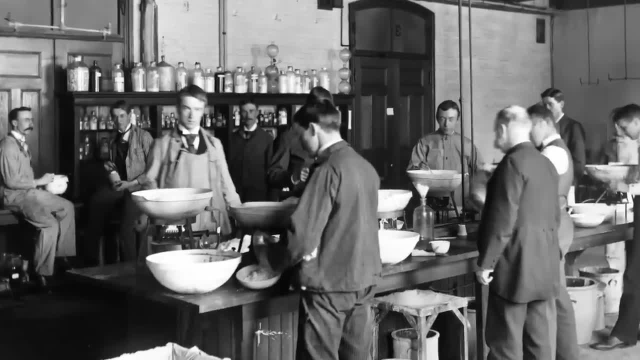 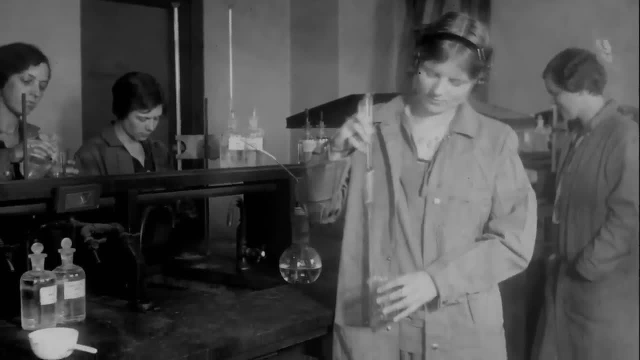 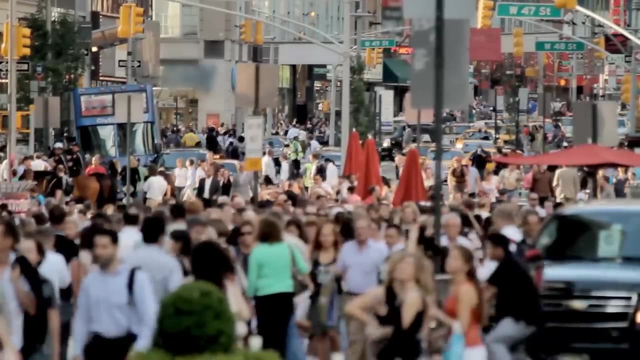 It was with this in mind that, in 1900,, in 1908, a group of chemical engineers who saw the promise in the future joined together with a mission to advance the profession and the society we serve Under the stewardship of AICHE. 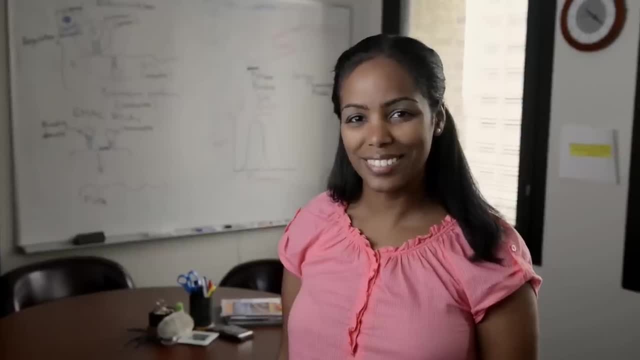 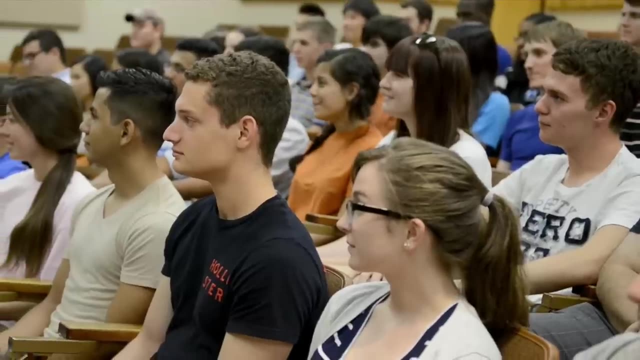 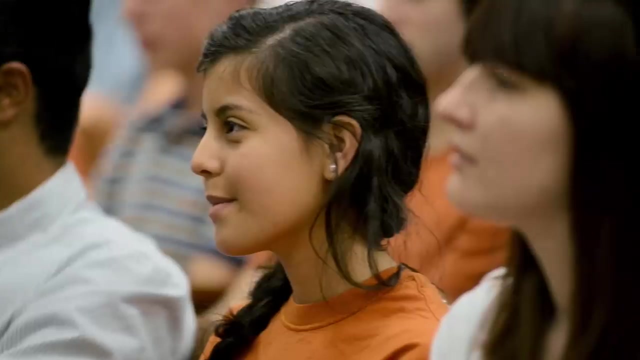 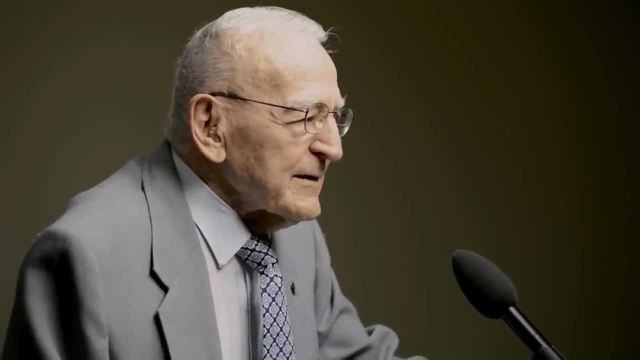 our profession is stronger, safer, better educated and more diverse. As we enter a new era of chemical engineering, new challenges, Our charge is perhaps greater now than at any time since our founding, for our mission is not only to protect our legacy, but to keep the